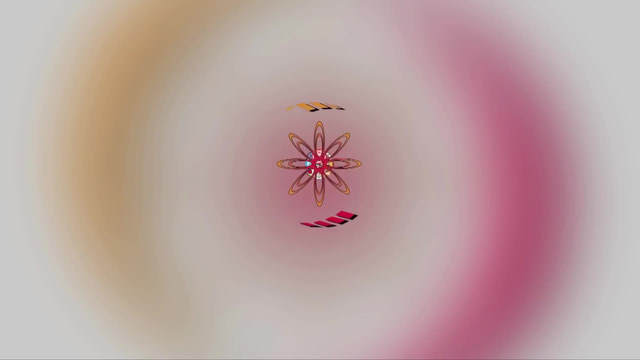 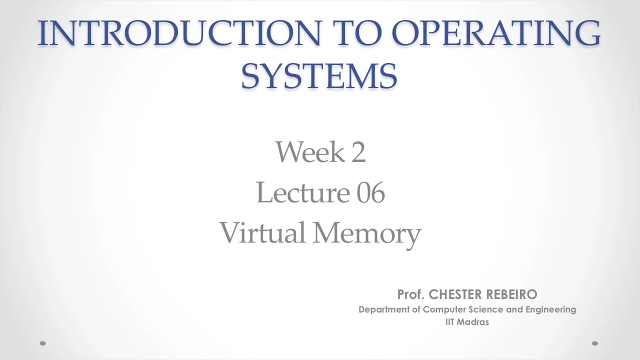 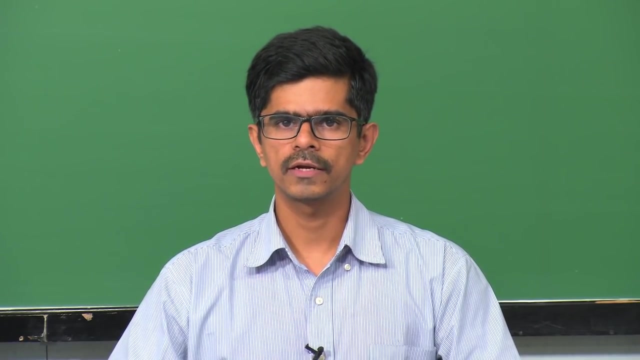 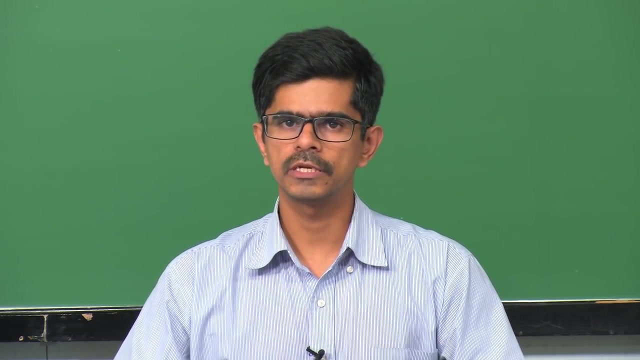 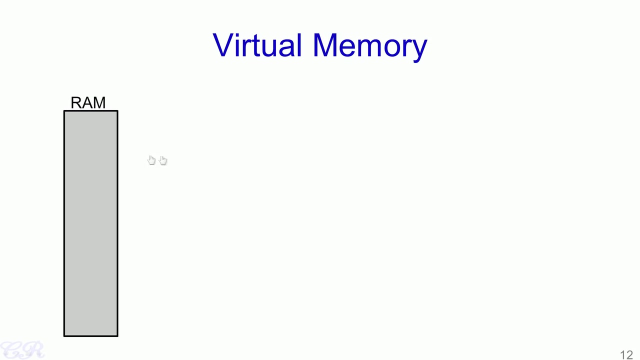 Hello, in this video we will look at Virtual Memory, which is by far the most commonly used memory management techniques in systems these days. So in a virtual memory system, the entire RAM which is present in the system is split into equal sized partitions, called. 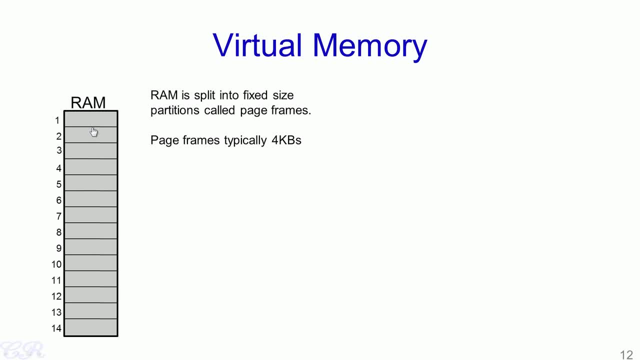 page frames. So typically page frames would be of 4 kilobytes each. So in this RAM, for instance, we have 14 page frames, Page frames which are numbered 1 to 14, and each of these page frames have the same size. 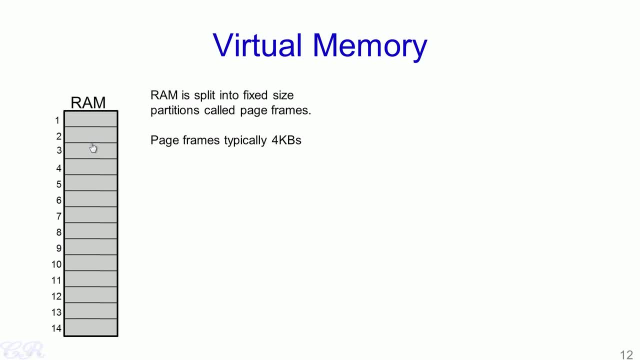 In the previous Intel processors all pages were fixed at 4 kilobytes, but in more recent processors we could have pages or page frames which are of a larger size. In a similar way, the process which executes in the CPU or the process 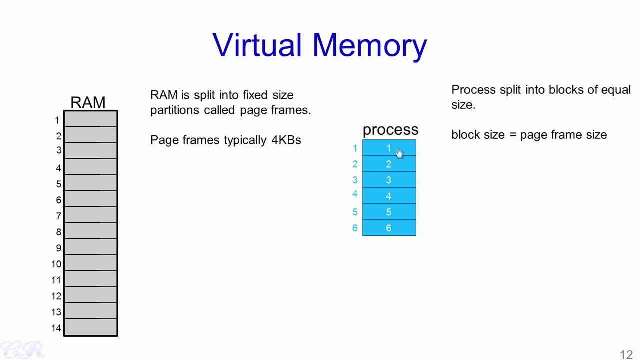 map corresponding to the process is also split into equal sized blocks. Now the split of a process is in such a way that the block size of a process, that is, this size, is equal to the page frame size. that is, the size of each block in this process is equal to the. 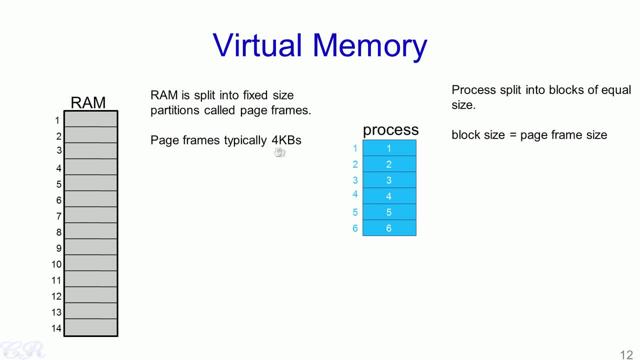 page frame size Now, because we have split the RAM like this, as well as the processes memory in a similar way. what we can then do is allocate blocks in a process to page frames in the RAM. Additionally, what the operating system maintains is a table. 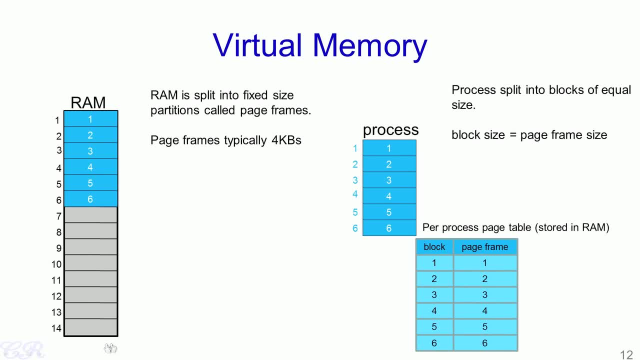 This table is also present in the RAM and not shown over here, But what it contains is the mapping from the process blocks to the page frames, For instance over here the mapping is very simple: Block 1 of the process gets mapped into page frame number 1, that 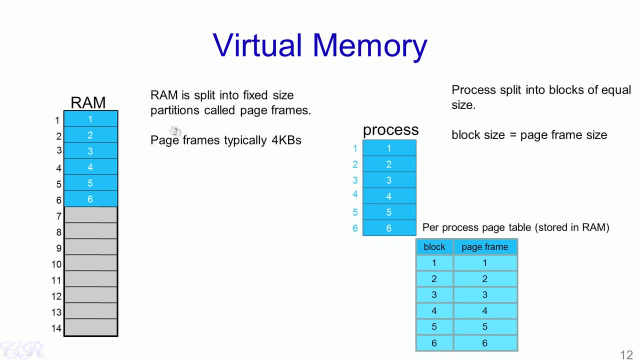 is block 1 of the process gets mapped into page frame number 1, block 2 gets mapped to page frame 2, block 3 gets mapped to page frame 3, and so on. Now this… I would like to highlight again is a per process page table. So per process means that every 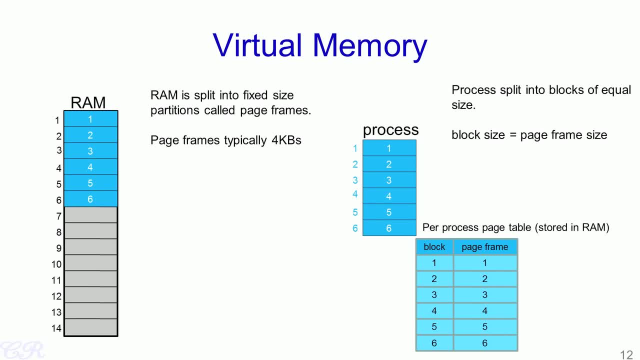 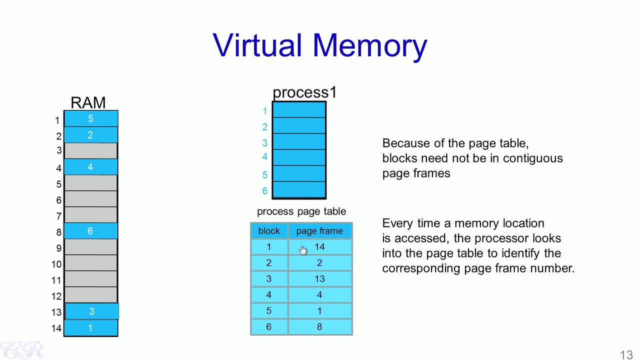 process running on the system will have a similar page table, as shown over here. Now, because we have such a table, which provides the mapping between blocks of a process to the corresponding page frame, what we can then do is…. So what we can do is we could have any kind of mapping that we choose, For instance now. 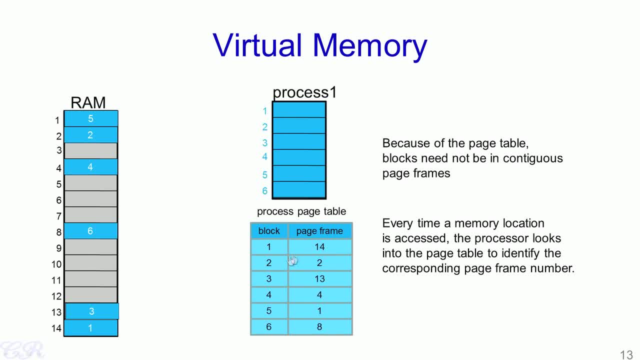 we have block 1 of the process present in block 14, that is over here- block 2 of the process present in page frame 2, block 3 of the process in page frame 13, and so on. Essentially, what we are able to achieve with this particular process page table is that 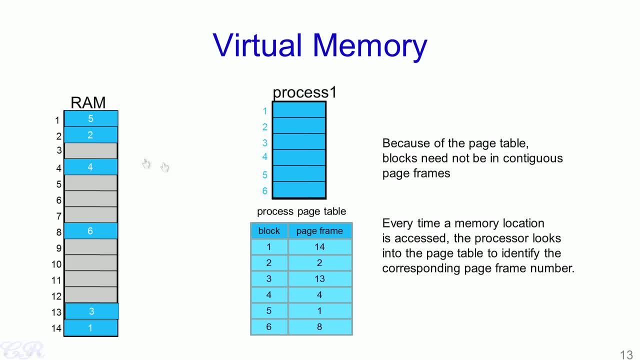 the blocks of the process may not be in contiguous page frames in the RAM. however, the overhead that we incur is that every time a particular memory location needs to be accessed in the processes memory map, the CPU would need to look up the processes page table, obtain the 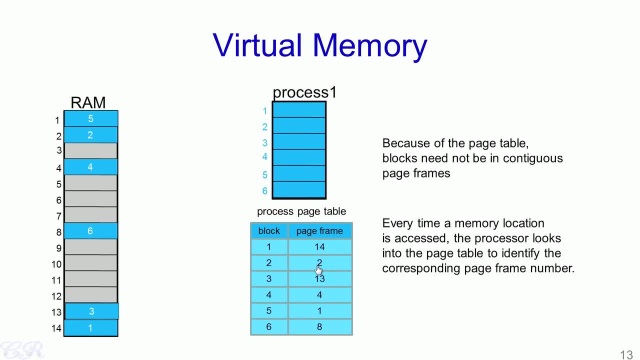 corresponding page frame data and입니다 the technique we are able to try this output frame number for that particular address, and only then can the RAM be addressed or accessed. For instance, let us say that the program executing in the CPU accesses a memory location. 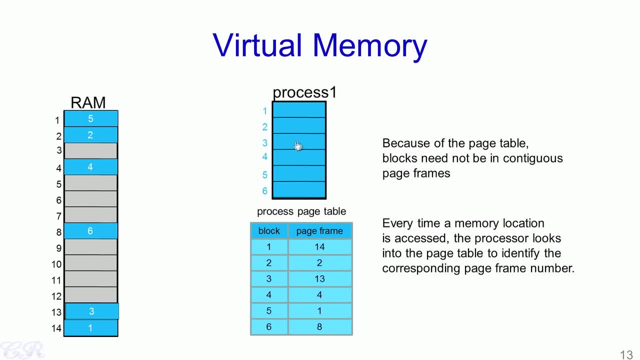 in, say, the block 3 of the process. So this could be an instruction or a load or store to some data. Now, when such an operation is executed, a memory management unit present in the processor would intercept this access and then it is going to look up into the page table and find. 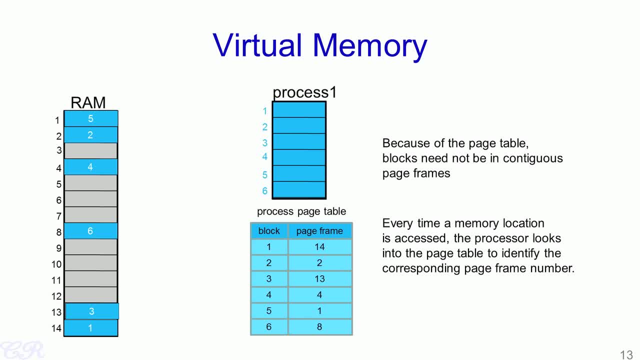 that the corresponding page frame which stores block number 3 is 13.. Then it is going to generate something known as a physical address, Which will then look into the 13th page frame in RAM. As a result, every memory access has the additional overhead of looking into the page table before. 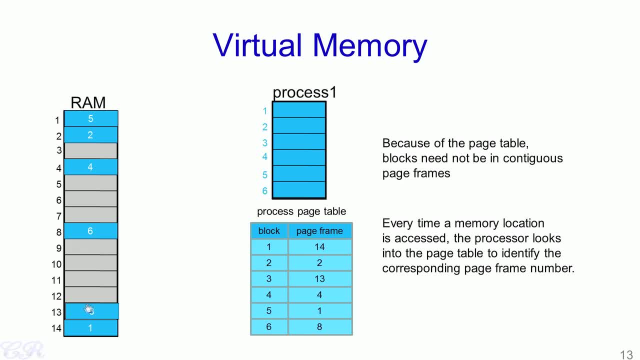 the access into RAM can be made possible. So this lookup into the page table is the extra overhead and typically this overhead is partially mitigated by using something known as a memory, A TLB cache or a translational look aside buffer cache. So we will not go into details about TLB cache but for our understanding with respect, 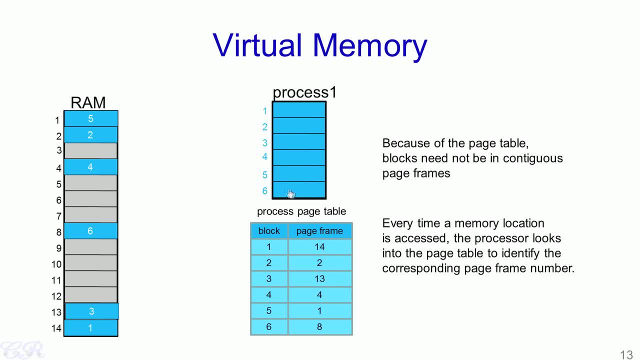 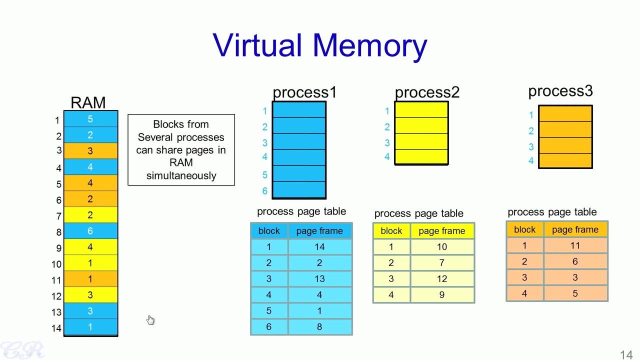 to the course we are studying. we need to remember that every memory access or every load or store or instruction fetched by the process during its execution would need to look up a particular page table, and only then can the RAM be accessed. Now, what we mentioned was that every process executing in the system would have its own. 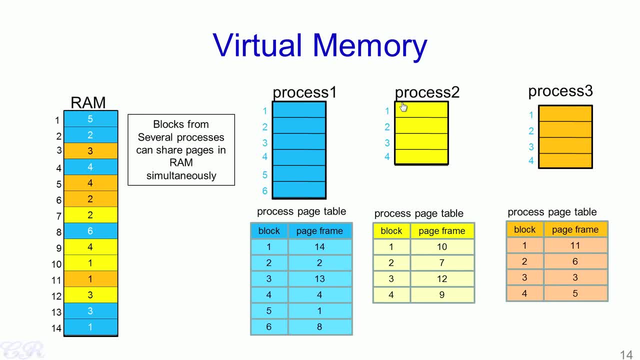 process page table. Thus, if you have a second process, that is, process 2, a process, 2 will also have its associated page table. Process 3 will also have its associated page table. Now, these processes or these processes, as we have seen the memory associated with these, 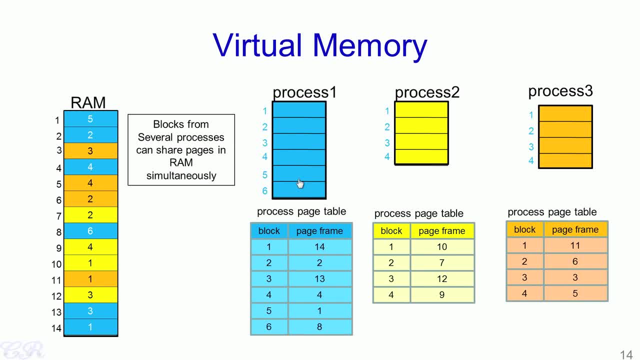 processes are present in the user space region of the memory. However, the process page tables are present in the kernel space and therefore any program you write in the user space would not be able to determine what the process page table mappings are. Now. since we have multiple processes executing in the system, each process could have various. 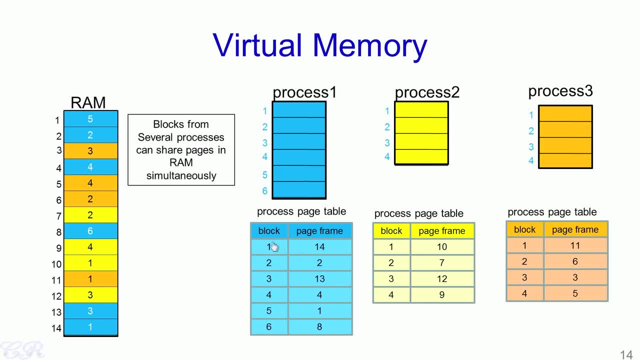 page frame mappings. For instance, process 1 has a mapping of all the blue page frames in this particular RAM, while process 2 has all the yellow page frames And process 3 has all the orange page frames. So now what we can see is that we are capable of sharing the RAM with multiple processes. 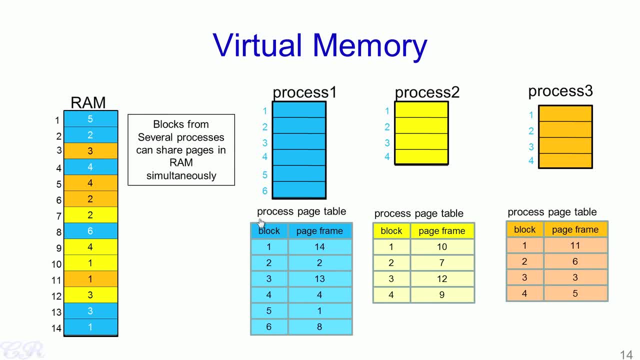 simultaneously. Now assume that we have a system with a single CPU. This means that at a particular point in time, only a single process will execute. process will continue to execute until its time slice completes, So during the execution of the process. that is when, for instance, process 1 is executing. 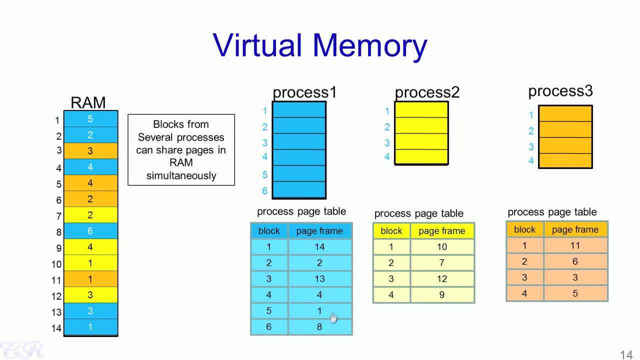 in the CPU, this particular process page table will be the active page table. Therefore, any instruction or data which is loaded or stored will look up this particular process page table to get the corresponding page frame in RAM. When there is a context switch from process 1 to say process 2, it would be this processes. 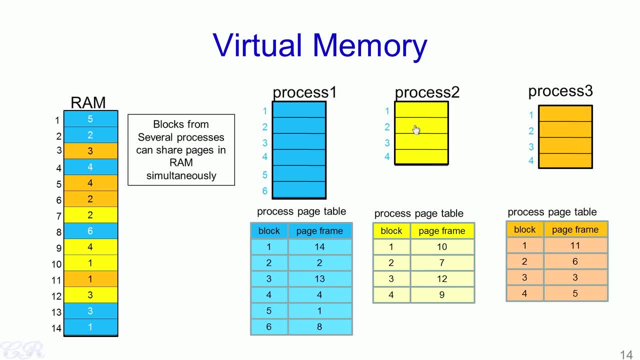 page table, which will become active. So any address that is accessed in process 2 will get the corresponding page frame number from this active page frame. Similarly, when process 3 is active, So process 3 gets executed in the CPU, this processes page table will be the active page. 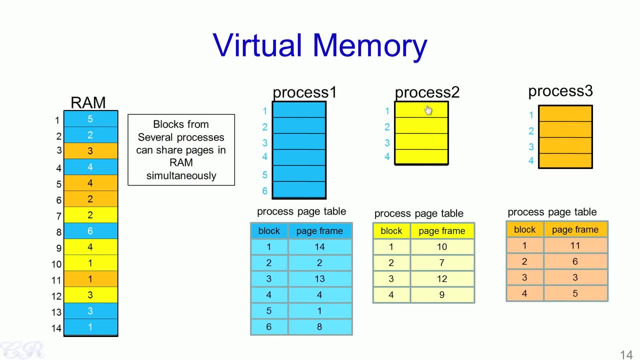 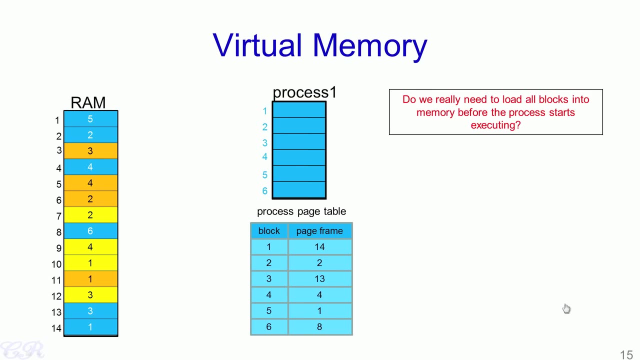 table. So what we can see is that it is not possible for process 2 to access any of the page frames corresponding to process 1 or process 3.. The next thing we would look at is that: do we really need to load all blocks? 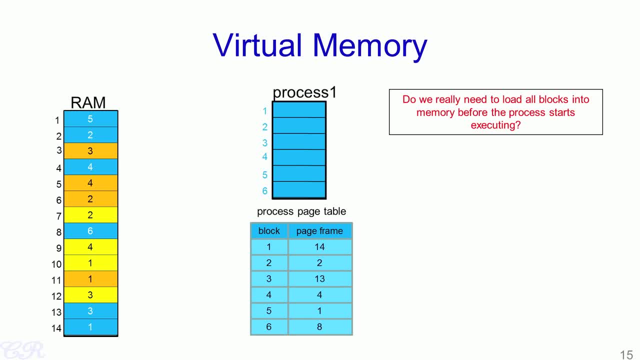 If we load blocks in the皇z-2 and process 2, how many blocks are removed? What is the load? How many blocks are we loading? In other words, in the previous video we had seen that when a process executes the entire, 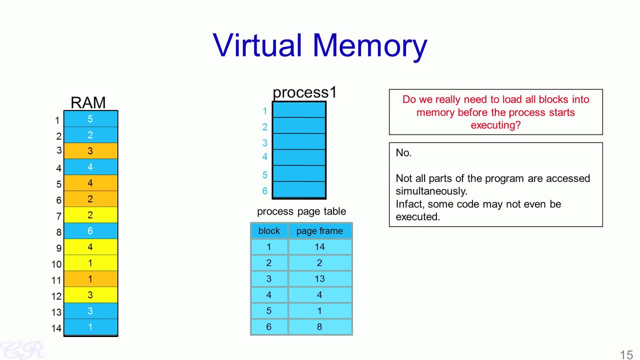 process was loaded into RAM. So now we ask ourselves that is such a loading actually required? and the answer is no. Essentially, what we notice about programs is that not all of the programs are loaded. Similarly, for example, for minigames, the loading time is recorded in students and the load time 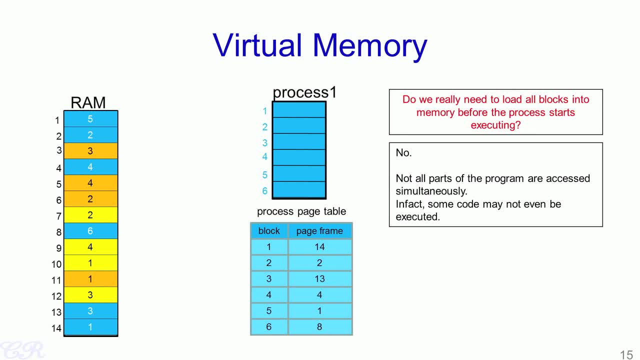 is recorded in that set of data. So when you load the program you do not get that all parts of the programs are accessed simultaneously. In other words, there is a locality aspect in the way a particular program executes. What this means is that if some instructions are executed in, let us say, this particular 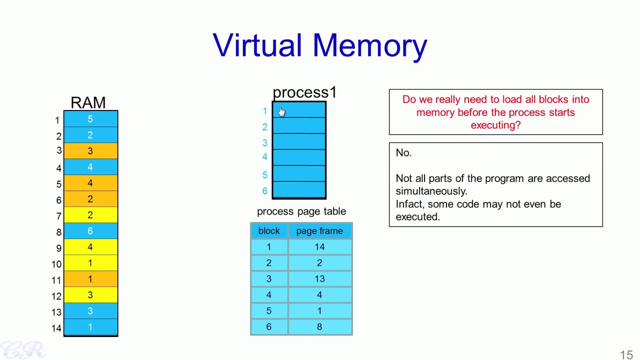 block, it is highly likely that the next set of instructions or the next few instructions that follow this would also be present in this block. So once there is a instruction to another block- say block 3, it is quite likely that because of the locality of the program, there would be quite a few instructions executed. 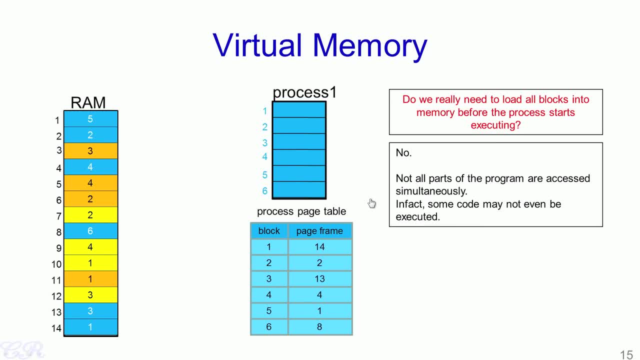 from this block, and so on. In fact, you may have- and it is quite often the case that there may be several parts of the process- memory Which are not even accessed at all, that is, they are neither executed, loaded or stored from memory. 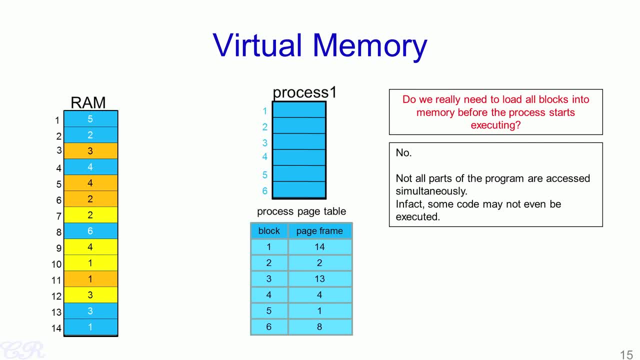 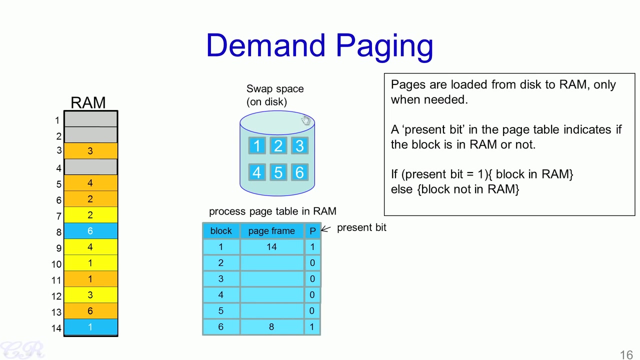 So what the virtual memory concept does is that it takes advantage of this locality aspect during the execution by using a concept known as demand paging. In a demand paging- So in a demand paging- what would happen is that we would have on a secondary storage 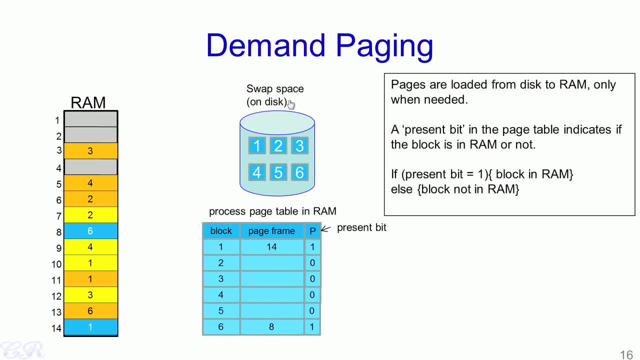 device like a hard disk, there would be a particular space allocated as the swap space. So in this swap space all blocks of the executable will be present. So for instance, if the process has 6 blocks, 1 to 6, and all the 6 blocks will be present. 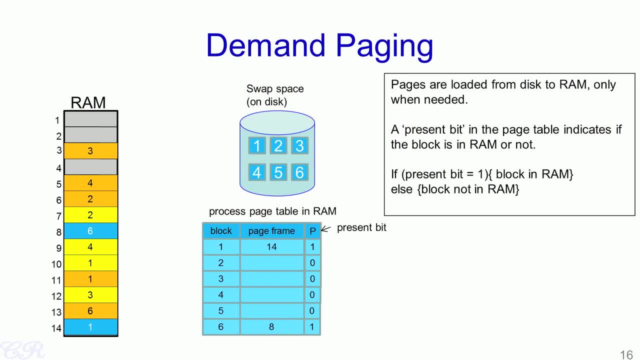 in the swap space, And only on demand will blocks be loaded from the swap space into the RAM. So now let us assume that there is an instruction which is executing in page frame 8 that corresponds to block 6 of the process, and it has resulted in a load or a store to a particular memory. 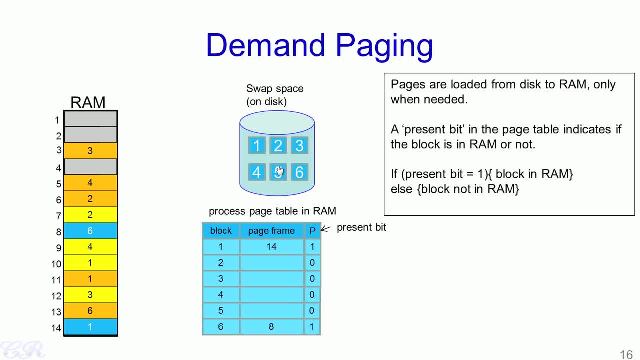 location In block number 5.. So what happens is that the processor is going to look up the process page table corresponding to block number 5 and see that the present bit is set to 0. So this would result in something known as a page fault trap, also called as the page. 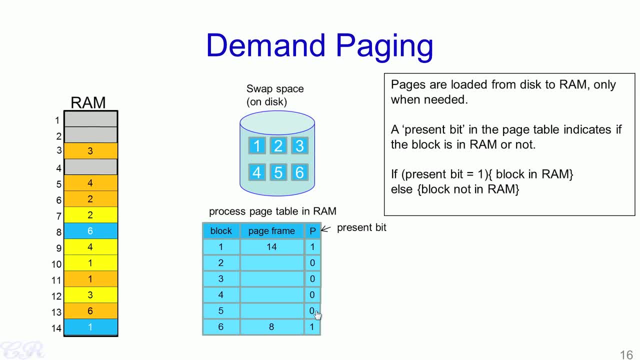 fault interrupt Now. the page fault interrupt would then trigger the operating system to execute Now. The operating system will then detect that this was a page fault interrupt and it will determine the cause of this page fault interrupt and it will load the corresponding page from. 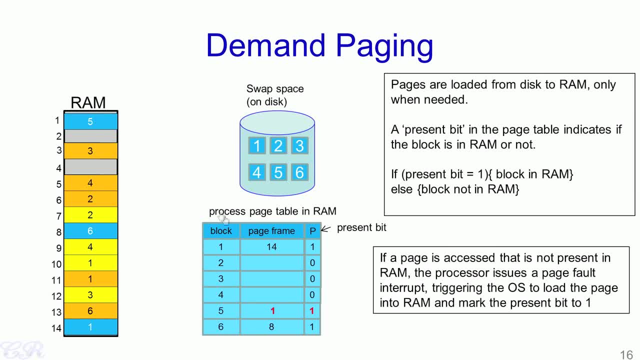 the disk into RAM. Consequently, it will also modify the processor's page table. For instance over here, a value of 1 is added to the page frame number and the present bit is set to 1.. Now, all later accesses to this particular block 5 will not cause a page fault, because 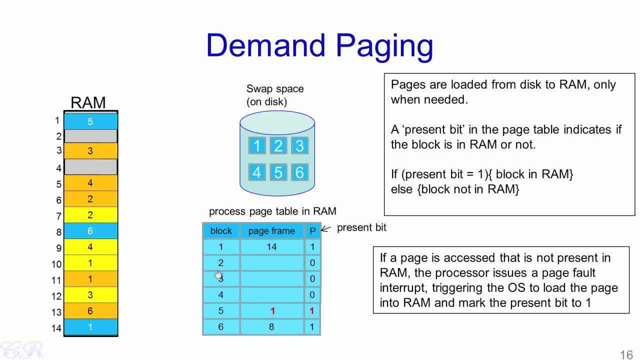 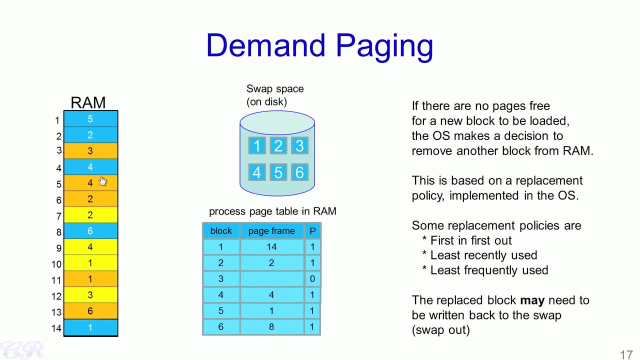 the present bit is set to 1.. However, the first accesses to block 2, 3 and 4 would result in page faults and it would cause the operating system to execute and load the corresponding blocks into the RAM. Consequently, The 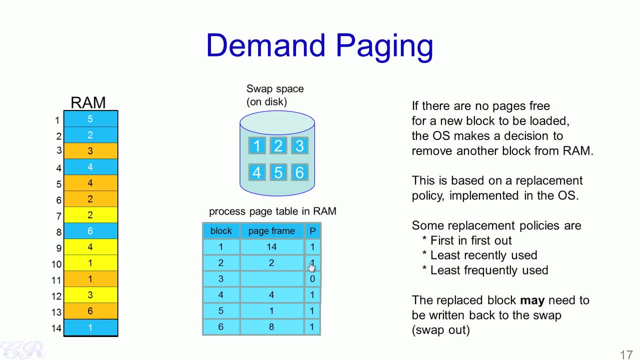 Page tables for that particular process will be updated. So now we have reached a state where every page frame in the RAM occupies some block. So this: these blocks could either be from the process 1 or process 2 or process 3.. Now what happens if, let us say, there is a memory access to process 1's RAM? 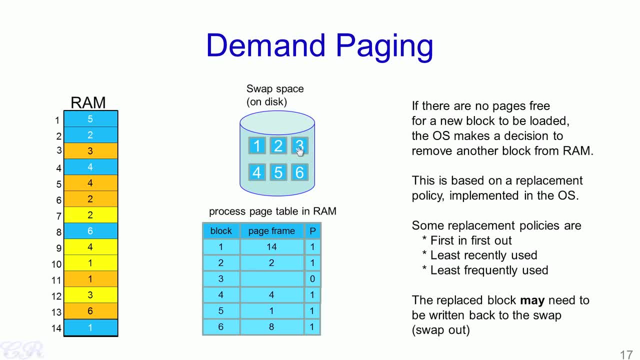 The memory access to process 1's third block. So as we can see that since the present bit is set to 0 in the process page table, it would result in a page fault interrupt that occurs and it would trigger the operating system to execute. 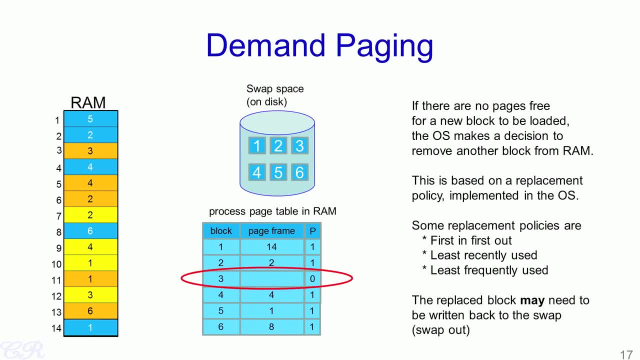 Now the thing is, what will the operating system do? So, in order to cater to this particular memory access in the third block, The operating system will execute the operating system. So, in order to cater to this particular memory access in the third block, The operating system would need to remove one of these pages. 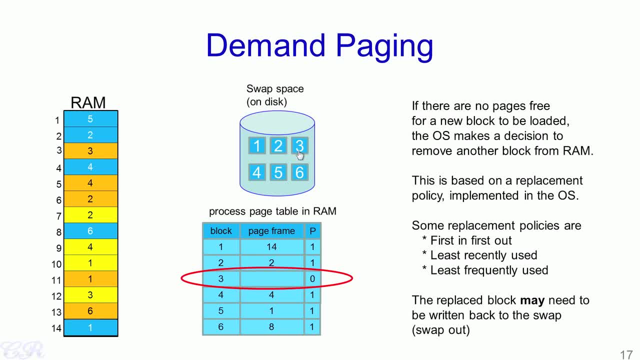 Essentially, it needs to clear up one of these page frames in order to make way for the new block. So the obvious decision that the operating system would need to make is which of these blocks should it remove in order to make way for the new block? 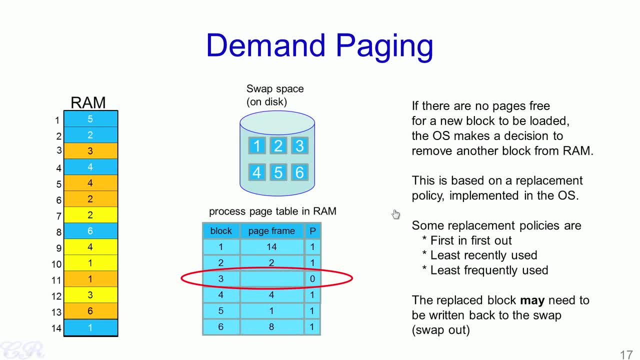 So this choice is based on sum. What are the Australok pouco引qang? so that means when we this количеisted, that company starts. It is now necessary for the other to go to some language to get this been removed. 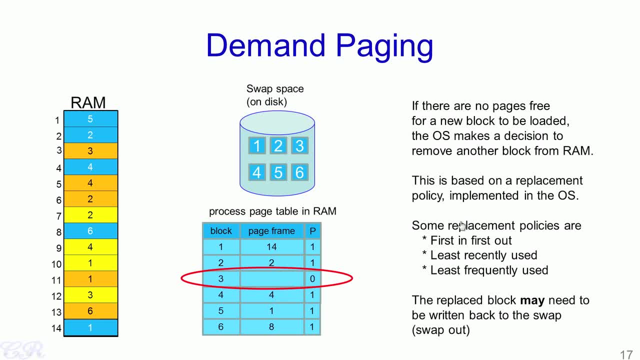 Now, as we have seen, lets say we are fully operating as the physical domain. it otherwise seems that it used a really vont same name. We can say that the work will start on Chernobyl. that's hit miserably and we will get faster. 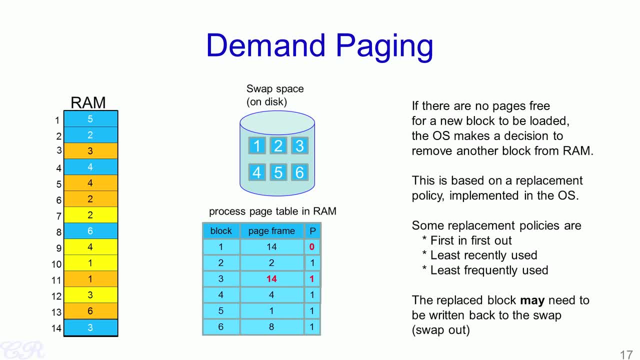 block that was recently accessed. Consequently, the present bit corresponding to the block that has been removed will be set to 0.. So we had removed, for instance, the block number 1 from the RAM to the swap and therefore the present bit corresponding to block 1 will be set to 0. 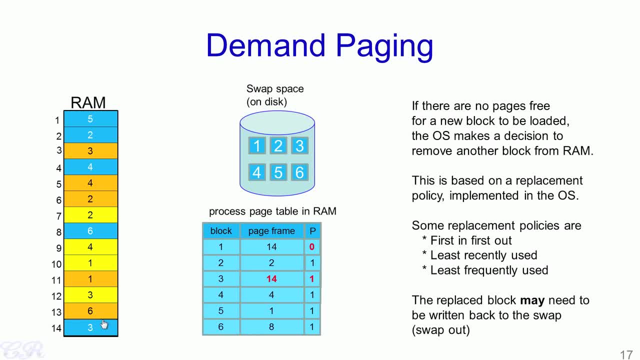 Now block 3, which has just got loaded into the particular page frame, will have its page frame number set and the present bit set to 1.. So this process of removing a block from the RAM and replacing it by another is known as the swap out and swap in, respectively. 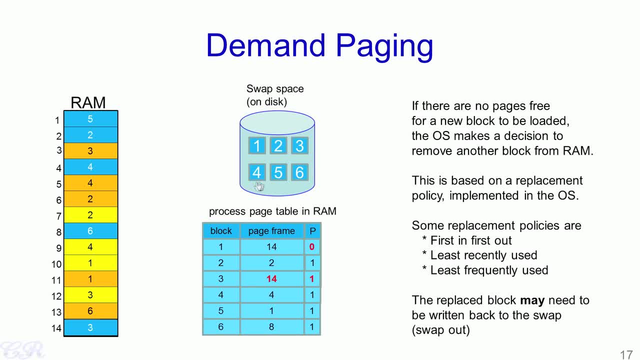 The process of moving a block So from the RAM to the disk is known as a swap out process, while the process of loading a block from the disk to the RAM is known as swap in. now, during the process of swap out, that is, storing block 1 to the hard disk. all though changes that happened during the 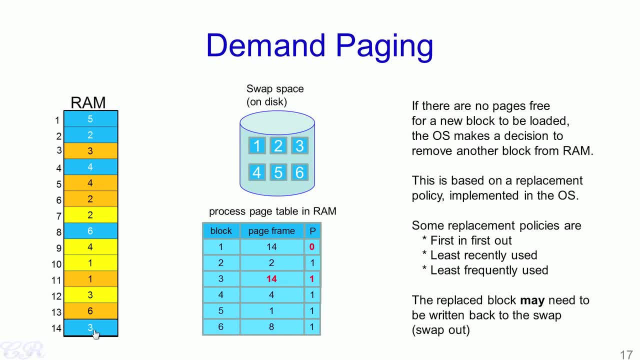 execution of the process, So this is called the swap out process. all changes that occurred in block 1 will get updated in the swap space. Thus the block which eventually gets stored in the swap space will have the latest view of the data. 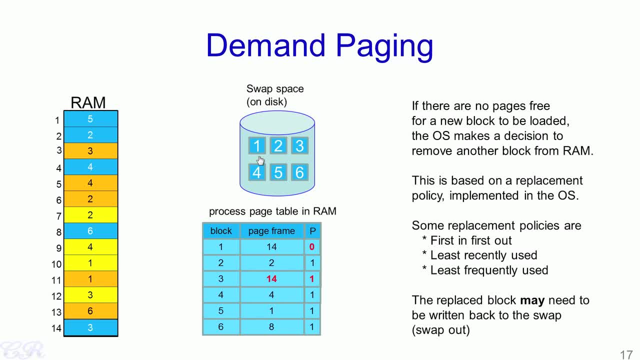 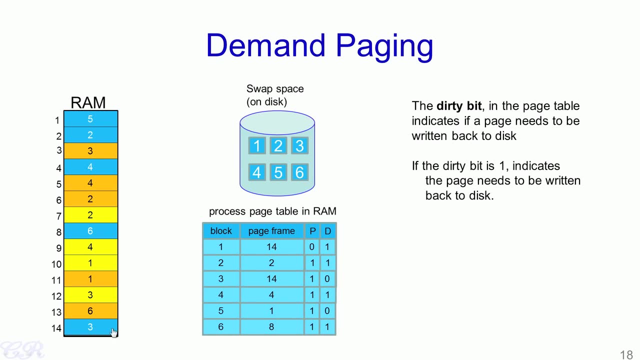 So the next thing that we are going to ask is that if the swap out, that is, the copying of the block 1 from the RAM to the disk, is actually required, Let us assume that block 1, which was present over here in the 14th frame, had no data that 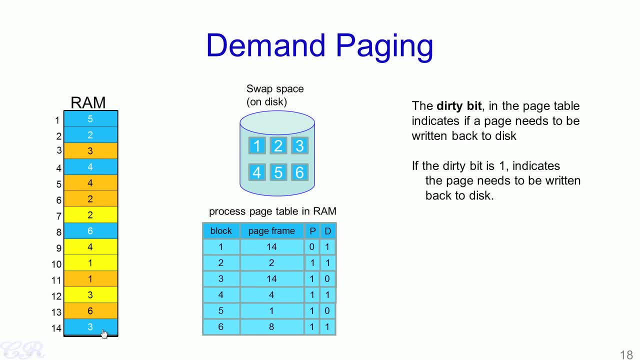 is changed. For instance, it could be corresponding to instructions or read-only data and therefore none of this data is changed. In such a case, the swap out process of copying the contents of this page frame back to the disk will not be required. 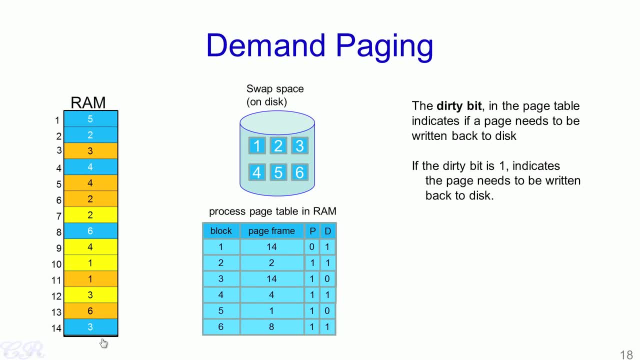 On the other hand, suppose we had data in block number 1 which was modified. So this would indicate that the copy of block 1 in the RAM is different from that in the disk And therefore the entire page frame should be swapped out and written back into the disk. 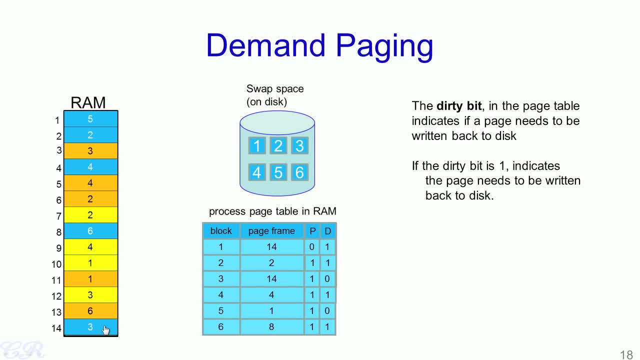 So how will the operating system know whether a swap out is required or not? So this is done by an additional bit which is present in the page table, known as the deep bit or the dirty bit. So the dirty bit essentially indicates whether the page frame is swapped out or not.